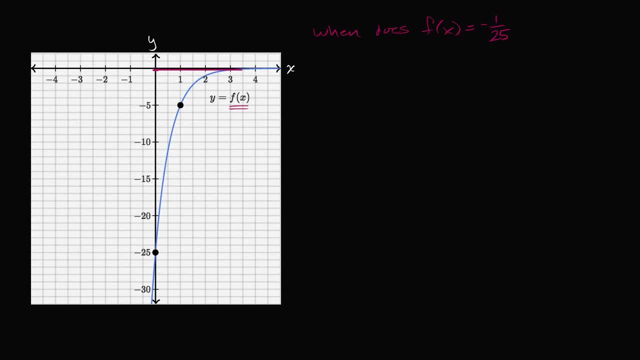 and then I can just solve for x. So let's do that. Well, since we know that f of x is an exponential function, we know it's gonna take the form. f of x is equal to our initial value a times our common ratio r to the xth power. 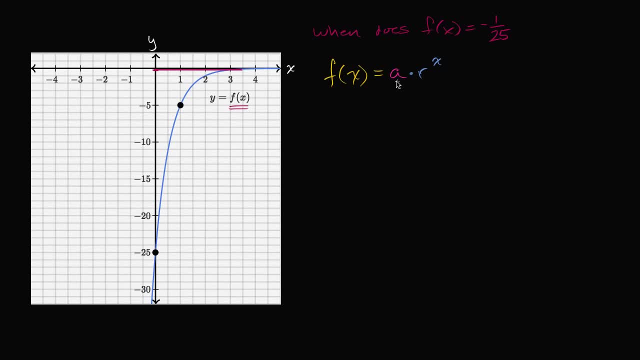 Well, the initial value is straightforward enough. That's going to be the value that the function takes on when x is equal to zero, And you can even see it here: If x is equal to zero, the r to the x would just be one. 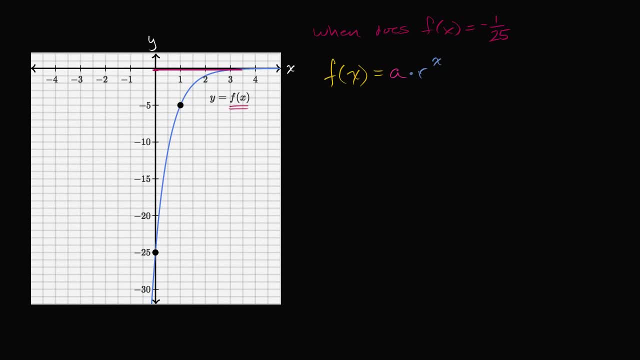 and so f of zero will just be equal to a. And so what is f of zero? Well, when x is equal to zero, this is essentially we're saying: where does it intersect? where does it intersect the y-axis? We see? f of zero is negative 25.. 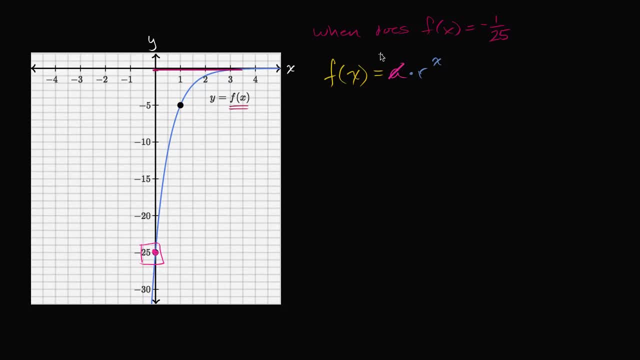 So a is going to be negative 25.. Negative 25.. When x is zero, the r to the x is just one. so f of zero is going to be negative 25.. We see that right over there. Now to figure out the common ratio: 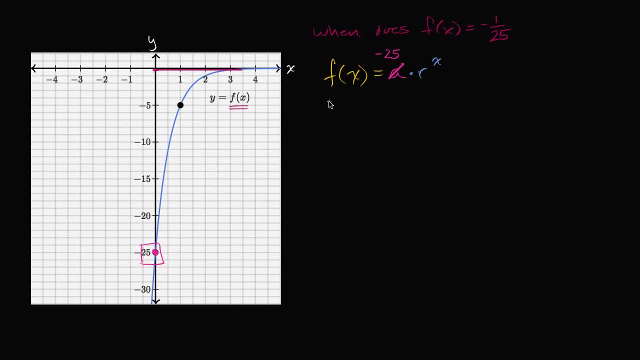 there's a couple of ways you could think about it. The common ratio is the ratio between two successive values that are separated by one. What do I mean by that? Well, you could view it as the ratio between f of one and f of zero. 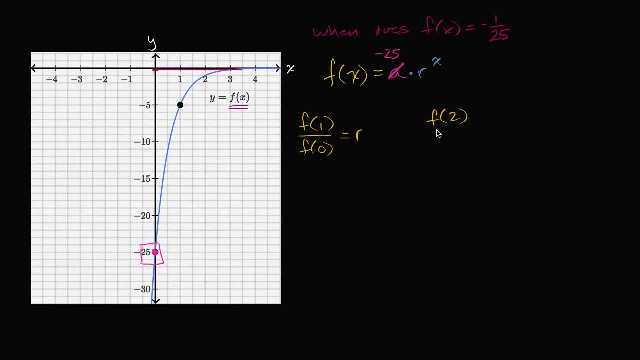 That's going to be the common ratio, Or the ratio between f of two and f of one. That is going to be the common ratio. Well, lucky for us, we know f of zero is negative 25, and we know that f of one 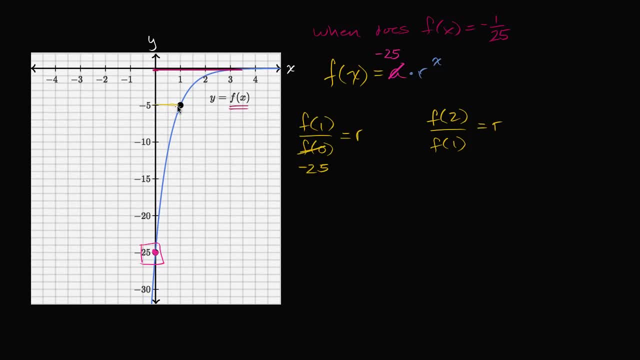 x is equal to one, y or f of x or f of one is equal to negative five, Negative five. And so, just like that, we're able to figure out that our common ratio r is negative five over negative 25, which is the same thing as 1: 5th. 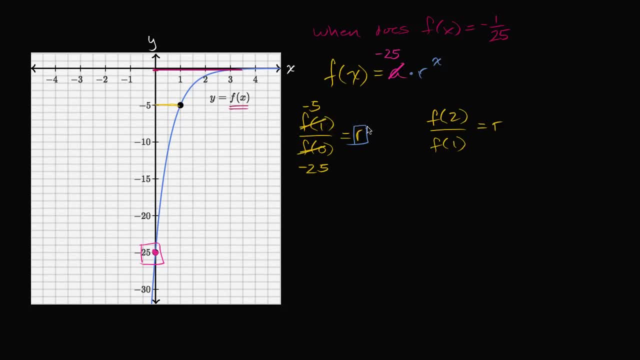 Divide a negative by a negative, you get a positive. So you're going to get five over 25, which is 1, 5th, Which is 1 5th. So now we can write an expression that defines f of x. 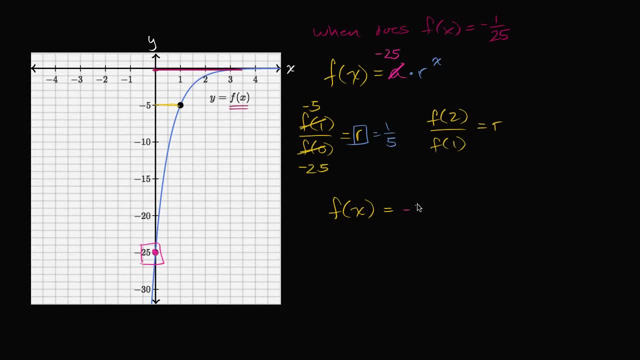 F of x is going to be equal to negative 25 times 1, 5th to the x power. And so let's go back to our question: When is this going to be equal to negative 1- 25th? So when does this equal to negative 1 25th? 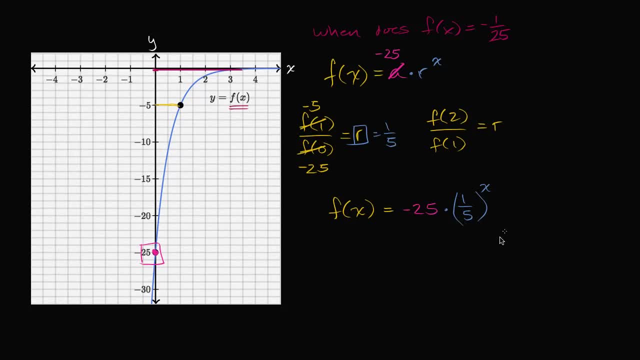 Well, let's just set them equal to each other. So let there's a siren outside. I don't know if you hear it So negative, I'll power through All right Negative. so let's see at what x value. 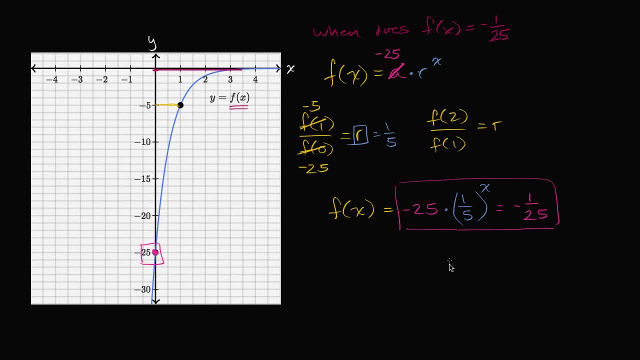 does this expression equal negative 1, 25th? Let's see, we can multiply. well, actually we want to solve for x. so let's see, let's divide both sides by negative 25.. And so we are going to get 1, 5th to the x power. 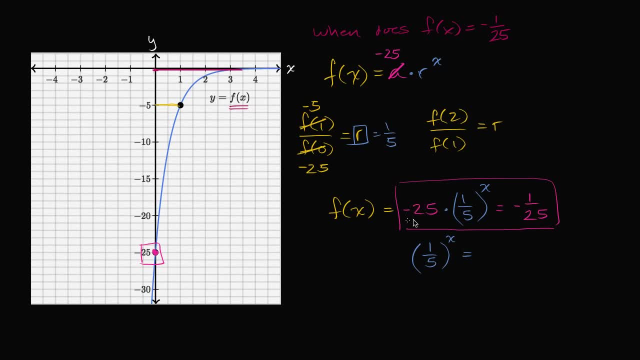 is equal to if we divide both sides by negative 25, this negative 25 is going to go away And on the right hand side, we're going to have divided negative by negative is going to be positive. It's going to be 1 over 625.. 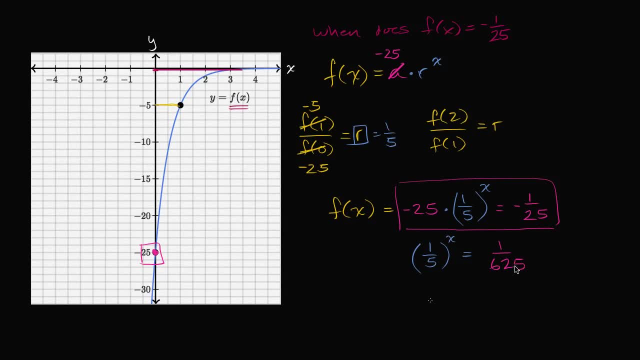 It's going to be 1 over 625.. And 1: 5th to the x power. this is the same thing as 1 to the x power over 5 to the x power is equal to 1 over 625.. 1 over 625.. 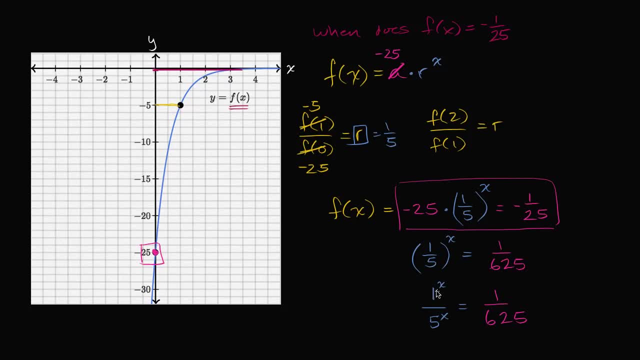 Well, 1 to the x power is just going to be equal to, is just going to be equal to 1.. So we could really it doesn't matter that we have this to the x power over here, And so we can see. I thought I was erasing that. 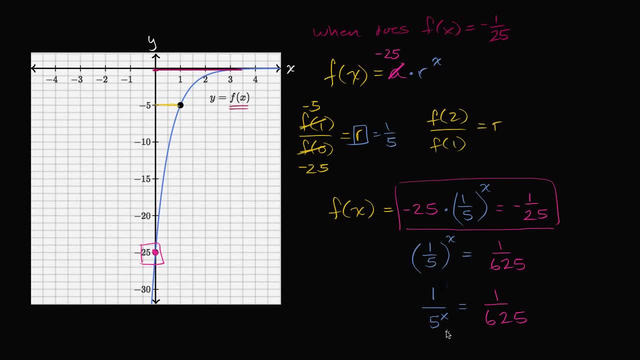 with a black color. there you go. That's a black color right over there, So we can see that 5 to the x power needs to be equal to 625.. So let me write that over here: 5, whoops, didn't change my color. 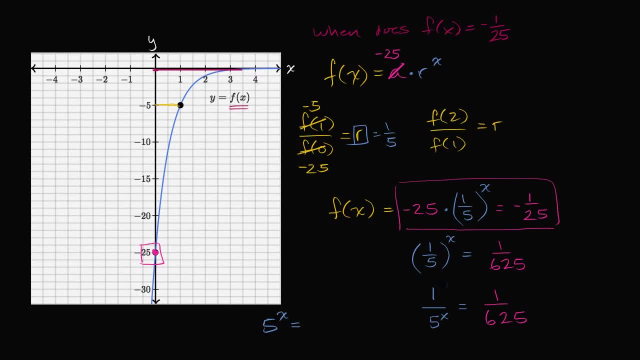 5 to the x, power needs to be equal to 625.. Now the best way I could think of doing this is: let's just think about our powers of 5.. So 5 to the 1st power is 5.. 5 squared is 25.. 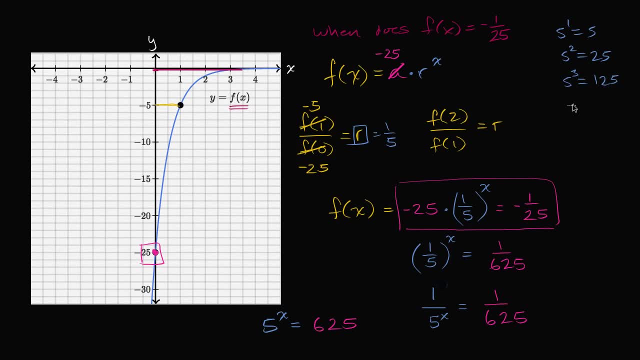 5 to the 3rd is 125.. 5 to the 4th: we'll multiply that by 5, you're going to get 625.. So x is going to be 4 is going to be 4,.